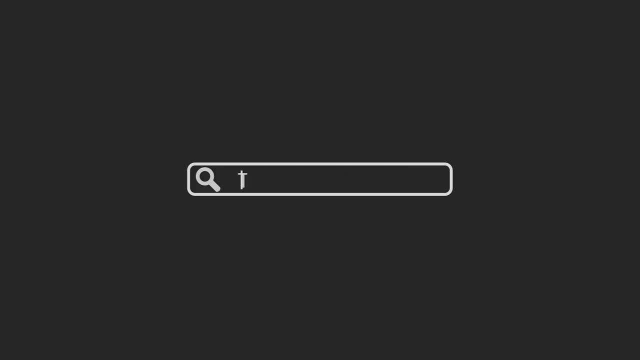 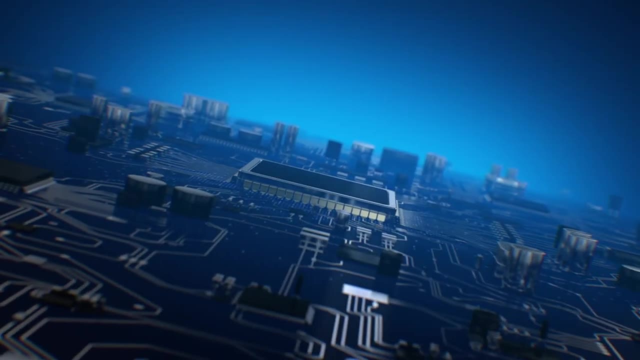 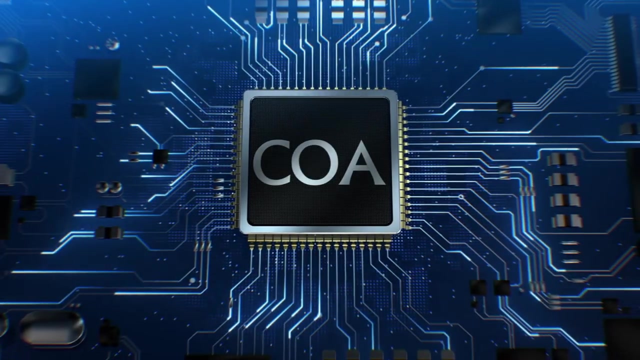 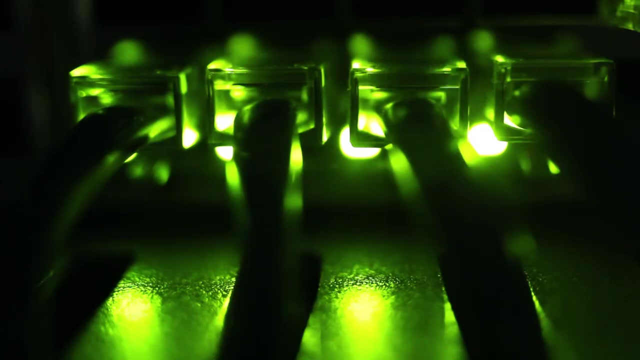 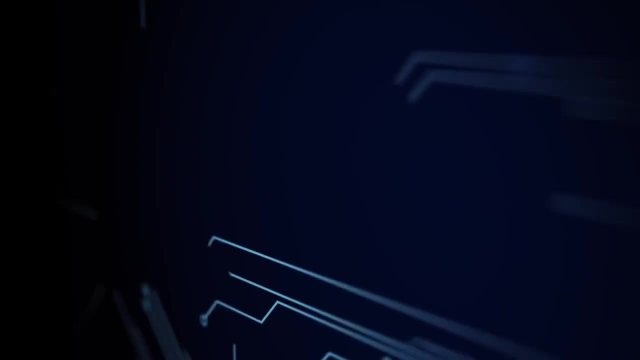 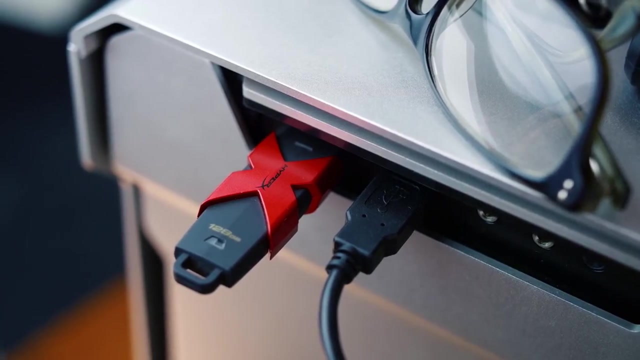 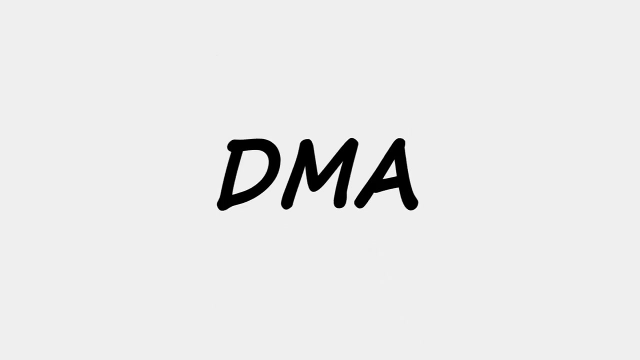 Have you ever thought how the data transfer works? How does your data from computer gets transferred to your peripheral device? How does your data from computer gets passed to a pen drive? Let's have a look. So, basically, DMA takes care of the entire data transfer operation. 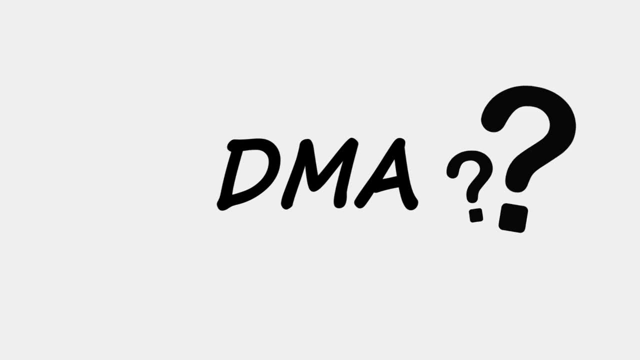 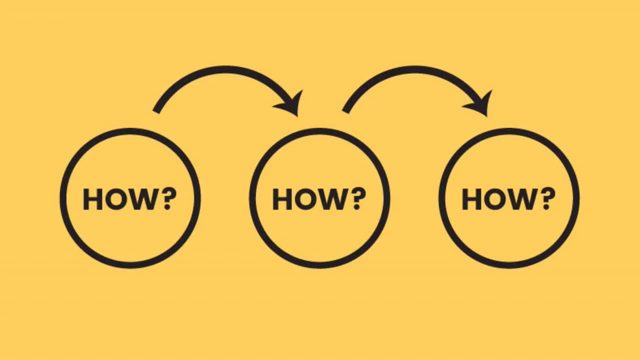 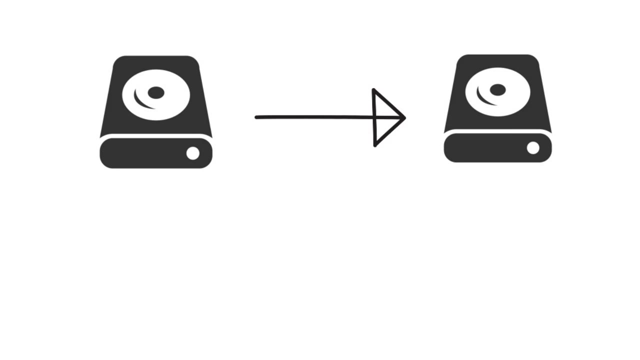 What does DMA stand for? DMA means Direct Memory Access. How does it perform the data transfer operation, You would wonder? In simple terms, DMA is an operation in which data is copied from one resource to another resource in a computer without the involvement of CPU. 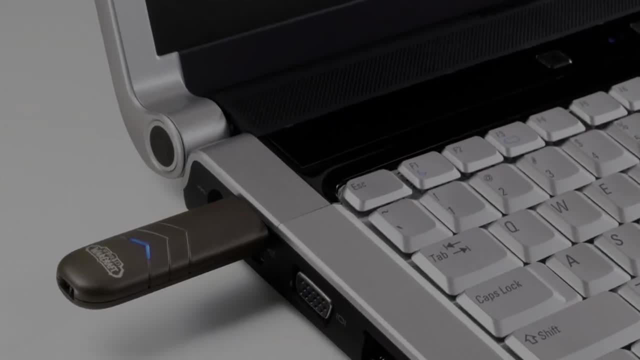 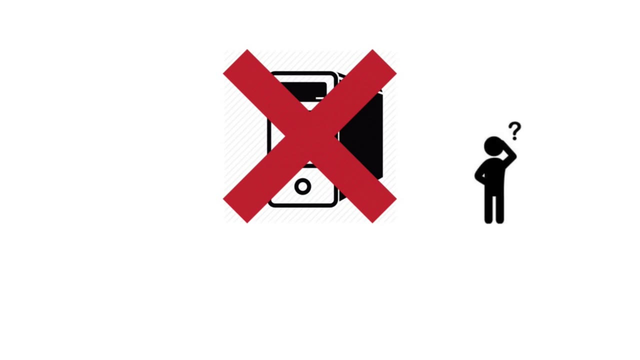 For example, the data from your computer memory to your external pen drive. You would ask: why without the involvement of CPU? Because CPU does the entire job. So why without the involvement of CPU? It is just to speed up the memory operations. 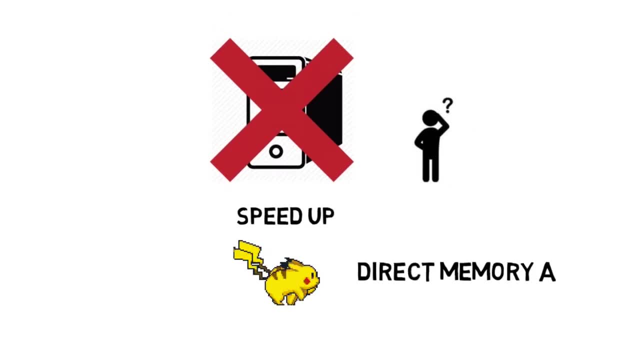 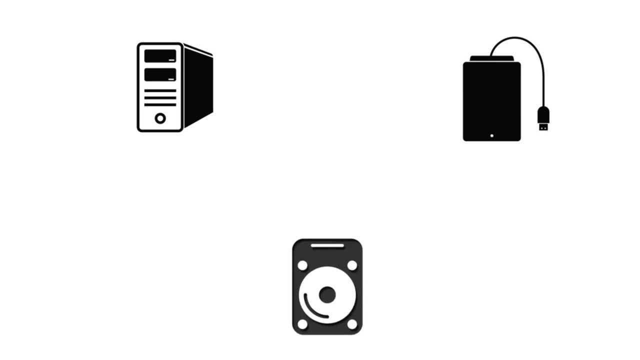 That's what it means: Direct Memory Access. Let us say we have a CPU, Input-output devices and the memory. Now, whenever we have to access memory, the input-output device goes to CPU and from CPU it goes to memory. So, as you can see, we need two cycles here. 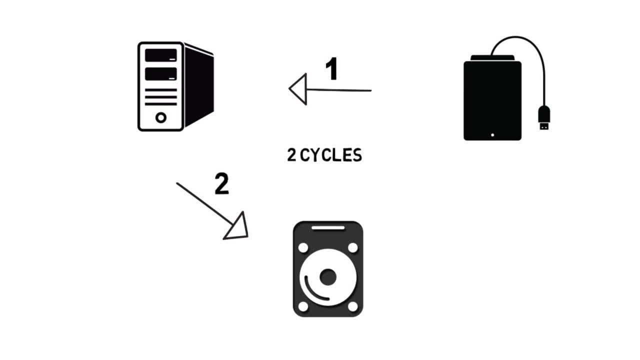 Since we need two cycles to perform this operation, the operation becomes complex and time consuming. Now let us say there is a direct connection from memory, or I mean from input-output, to memory. If this happens, the entire process can be completed in one cycle. 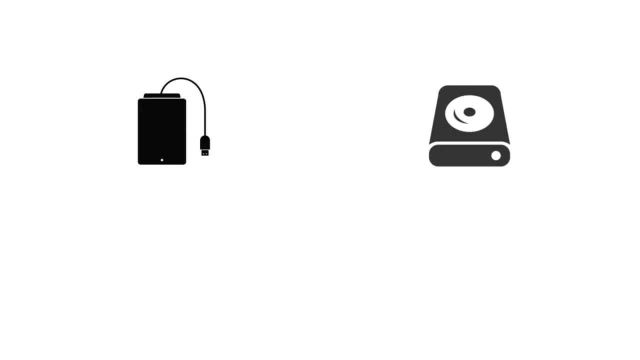 To provide this functionality, DMA was introduced. Here comes the rule of DMA. This connection between input-output to memory is provided by DMA controller, also known as DMASC. That's basically the short form of it. So this DMAC is the main chip that controls the entire DMA process. 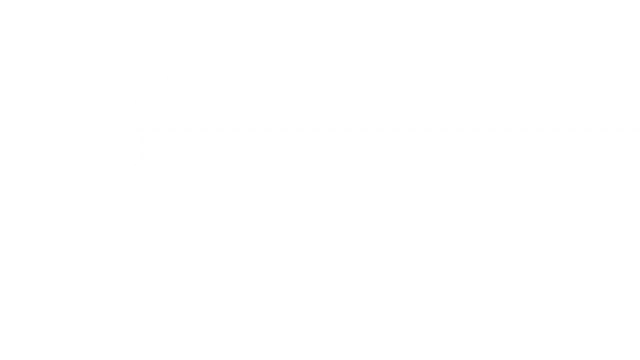 Let's see the working of this now. Okay, So first there is a CPU, Second we have DMA controller, Disk controller, And last we have the memory. As you can see, there are four blocks, And all these four blocks are connected to each other. 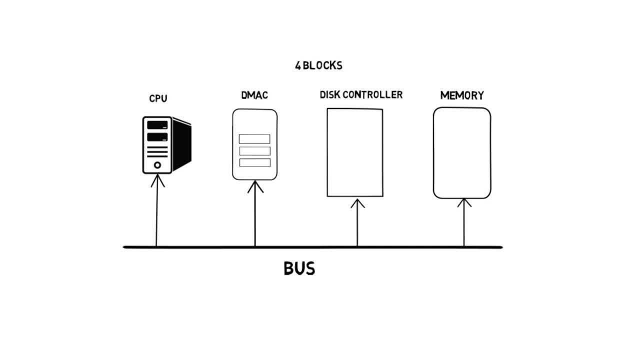 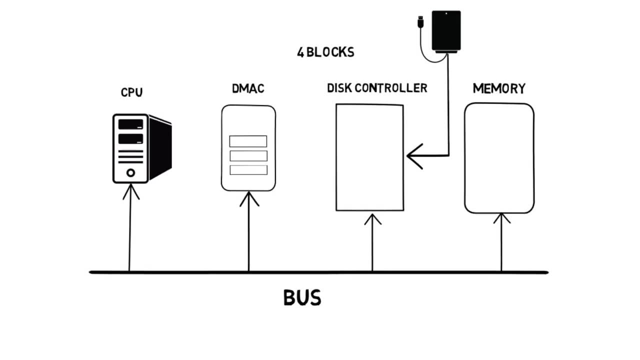 With the help of buses. Let's also add an external drive so that it becomes clear for better understanding. So basically, this is the overview of the entire DMA transfer operation. Now let's see how it actually performs the operation. So, firstly, what CPU does? is it programs the DMA controller by setting up its registers. 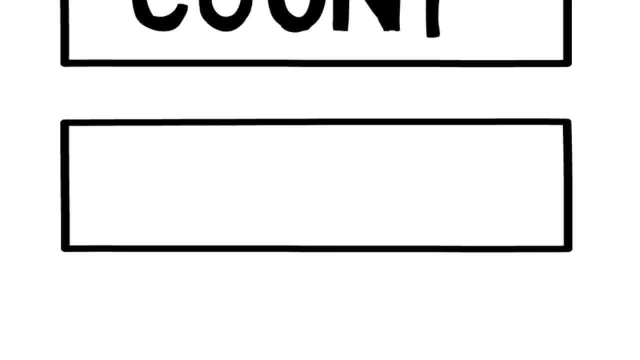 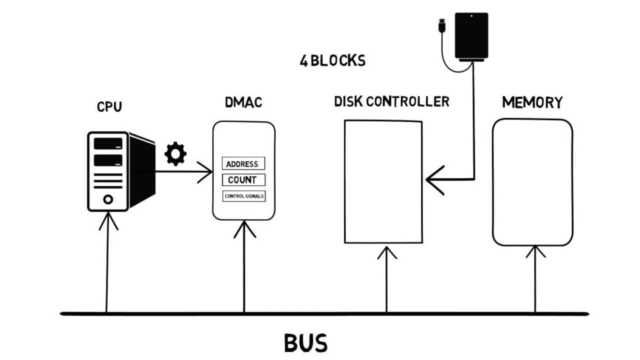 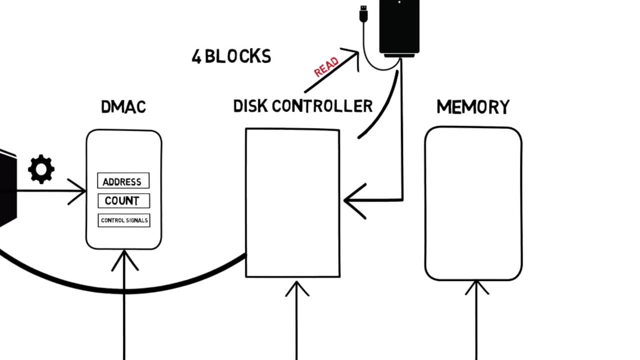 So this is the address, This is the count, These are the control signals. You will know its operation later. So what CPU does is it contacts the disk controller and instructs it to read the data from the external drive And store this data inside the internal buffer. 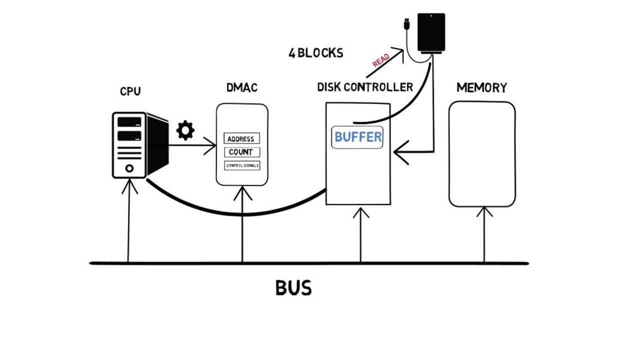 Here you can see we are using buffer. So why is it necessary to store the data into a buffer? So always remember: buffer is just a temporary storage unit in which we can store the data temporarily. The reason for using a buffer is because 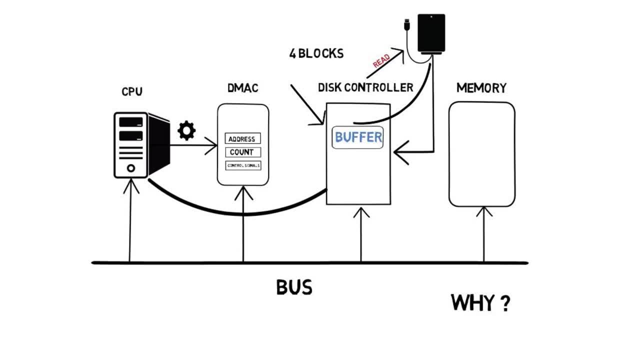 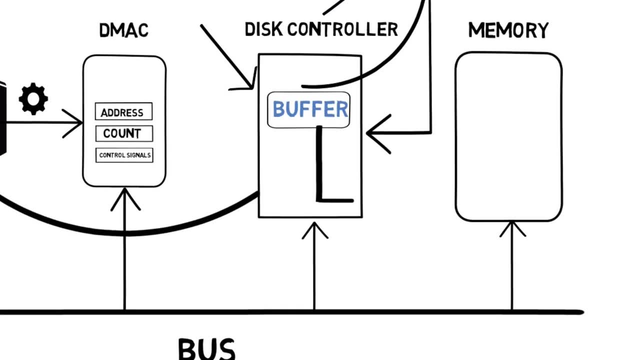 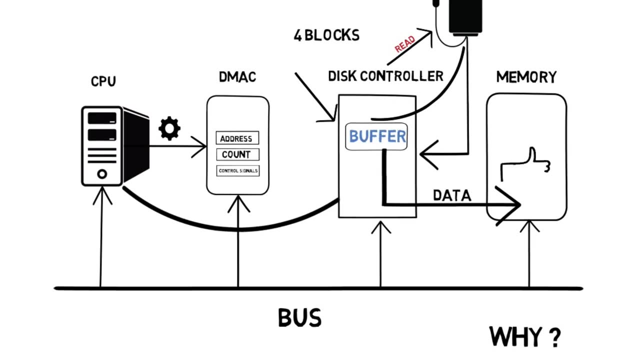 the DMA cannot perform its operation unless there is data inside a buffer. Okay, Now the next step is that the DMA controller will request disk controller to transfer the data which is in the buffer to the memory. So, whatever, the data that is present in the buffer will get transferred to the memory. 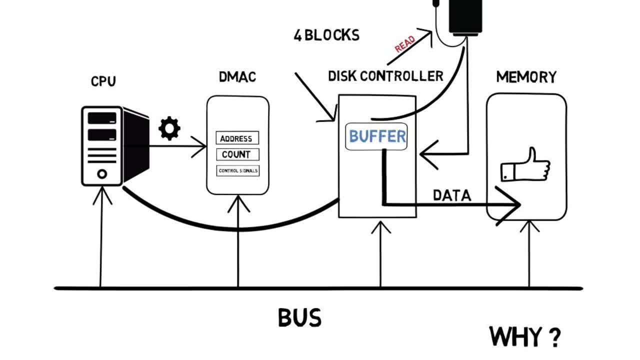 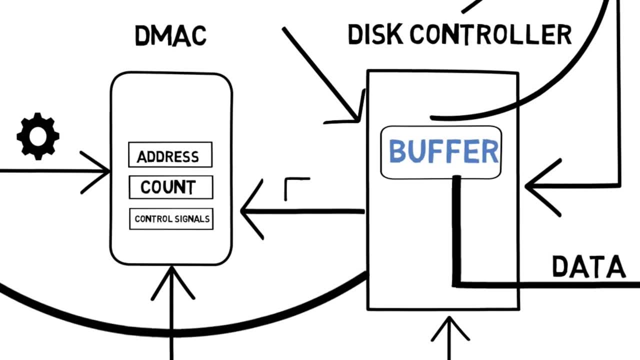 So, therefore, as how the disk controller was instructed, it will transfer the data into the memory. Once the first set of data is transferred, disk controller sends an acknowledgement to the DMA controller, stating it that it has finished the job that was assigned to it. 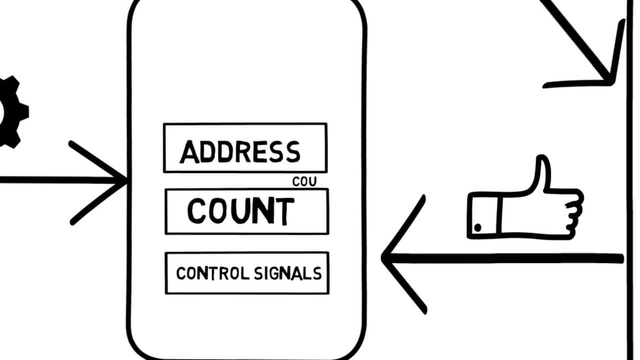 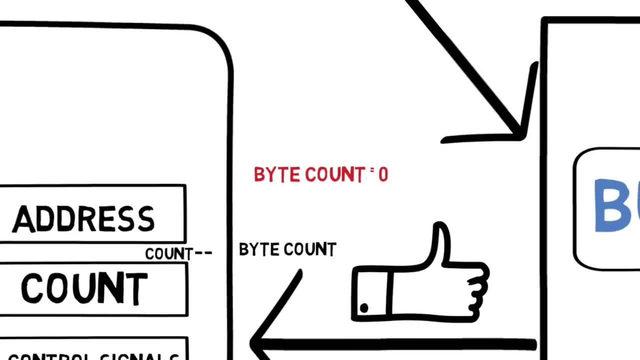 Once the DMA gets the acknowledgement, it decreases the count. This is known as byte count. Now the DMA will check if byte count is equals to 0. If it equals to 0, that means there is no more data that has to be sent.